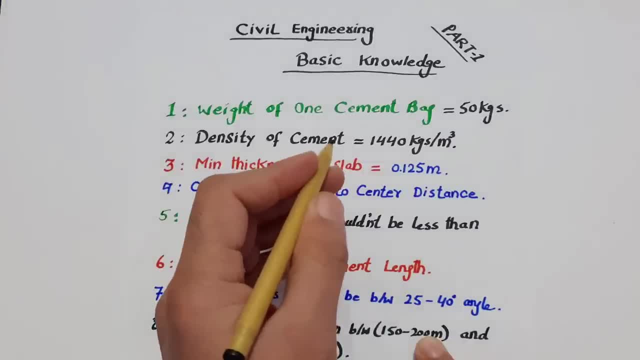 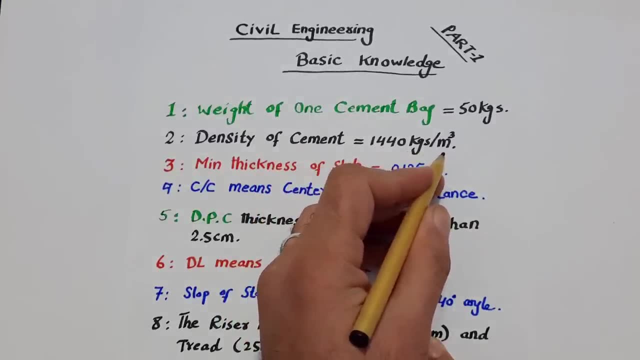 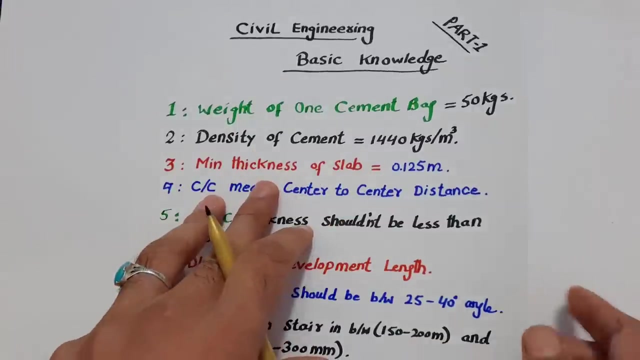 of cement. okay, so the density of cement is in meter cube or in cubic meter. that is 1440 kgs per meter cube. this is density of cement, okay. the third one is, guys, minimum thickness of slip. guys, we have about 15 points, okay, as you can see till. 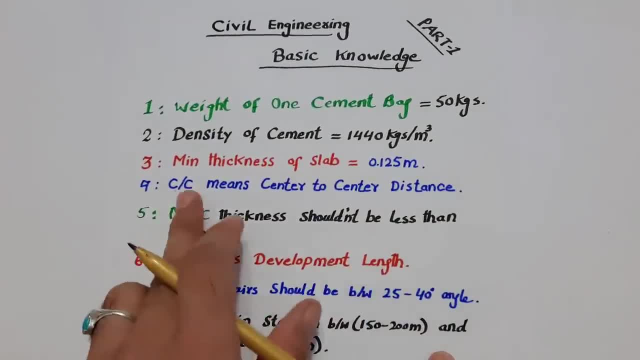 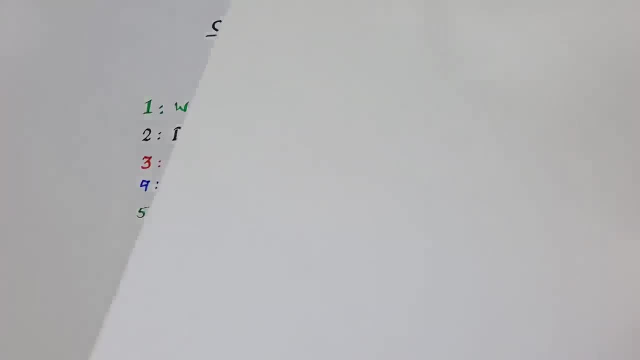 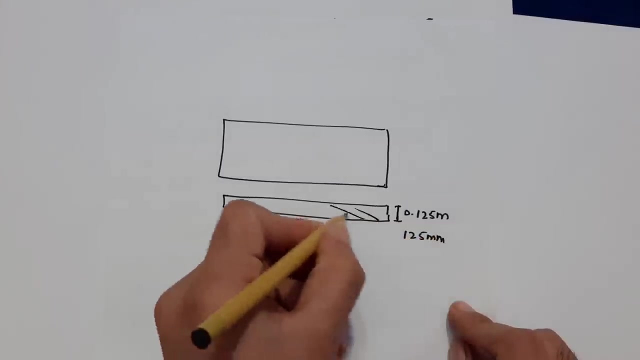 15. we have all right. the third one is minimum thickness of the slip. how minimum thickness of this? guys you can see here, this is top slip, okay, and, guys you can see, this is the section cross section. so the thickness of the slip should be minimum 0.125 meter or 125 millimeters. okay, thickness of 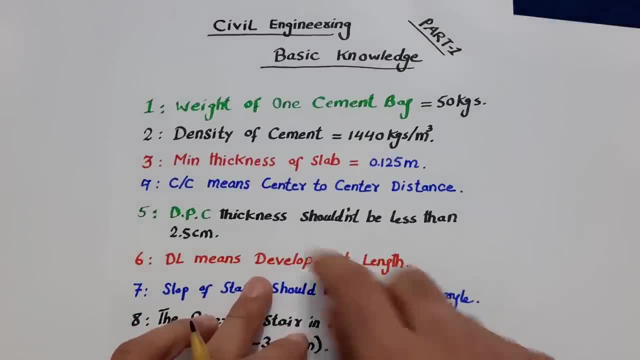 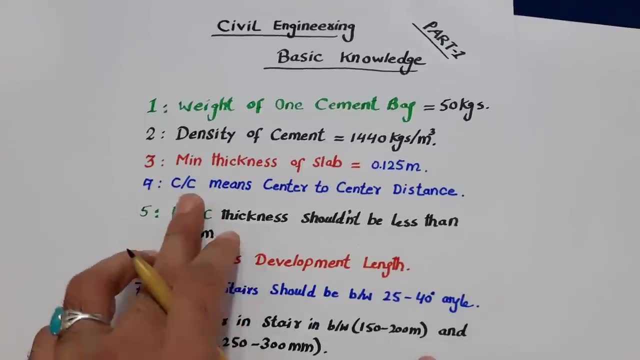 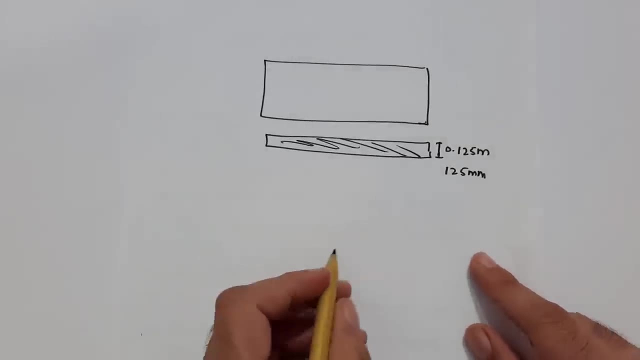 slip, okay, minimum. next, guys you can see. the fourth one is C slash C means central to central distance. okay, so C slash C especially we are using in steel structure QC, Hygood, so this isен design for the slab. are for any member, RCC members, like, guys you can see, this is the slab, so we are. 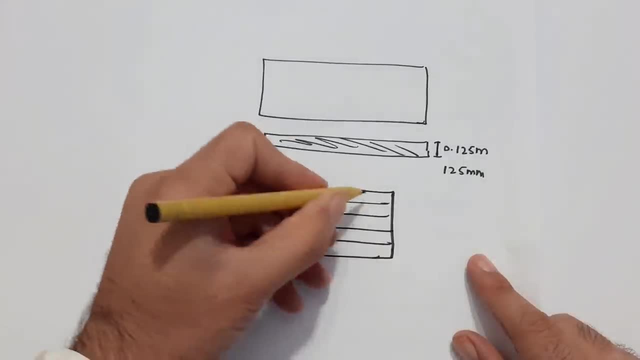 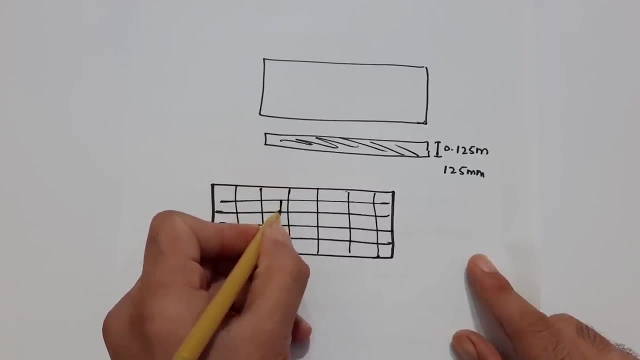 providing main bars and distribution bars. okay, guys, you can see these are distribution bars and these are main bars. okay, so the space between two steel rods, so we can say C slash C, for example six inches, ok. are C slash C? mean distance, QC, Hygood and ο Suppose these basketballs don't have an exact number. so we can say C slash C means they are six inches, okay. or C slash X, mioh. 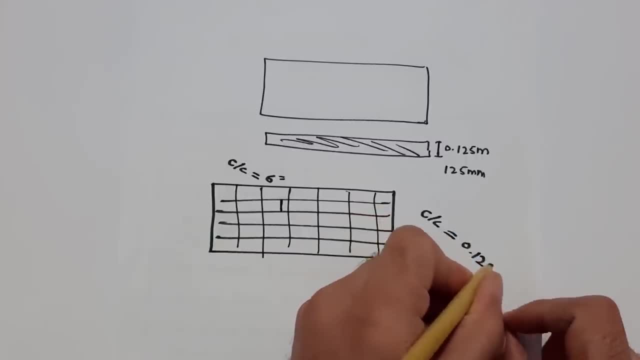 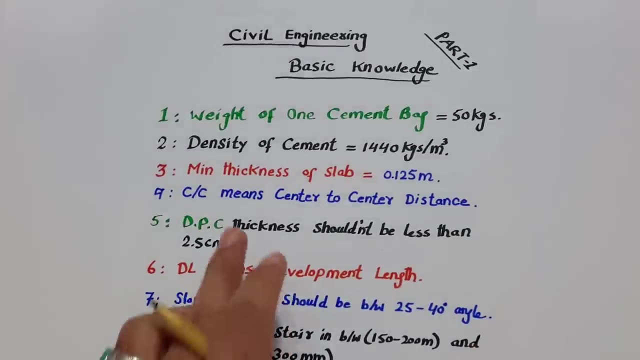 C is equal 0.125 meter, etc. okay, so it means spacing between two steel rods. okay, next one, guys, you can see thickness of DPC- damn proof course- which should not be less than 2.5 centimeter, are one inch right. the sixth one is, guys, DL means 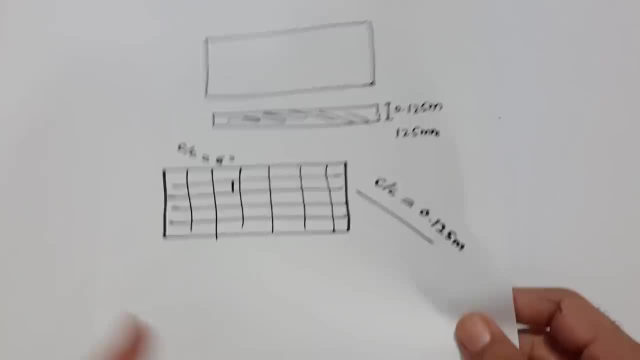 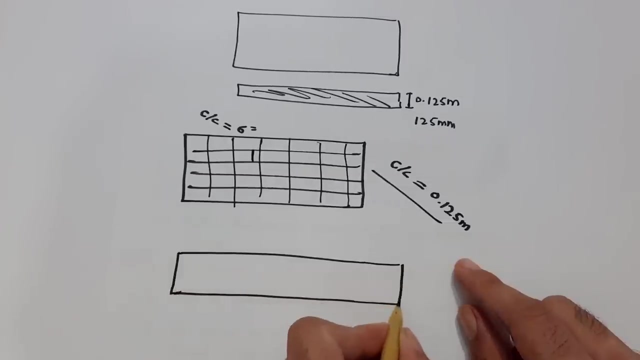 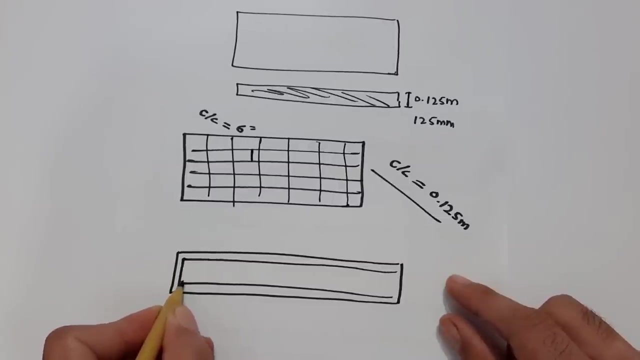 development length. what is development length, guys? you can see here this is beam, okay, so inside this beam I am providing the steel rods, okay, in long section. so, guys, you can see these are steel rods, okay. so this one still is coming to the downside and this one is going to the upward side. so, guys, this 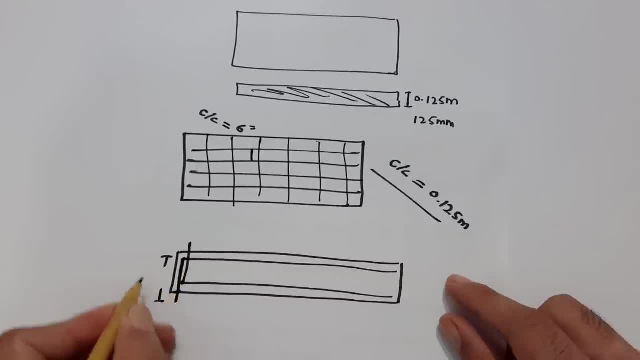 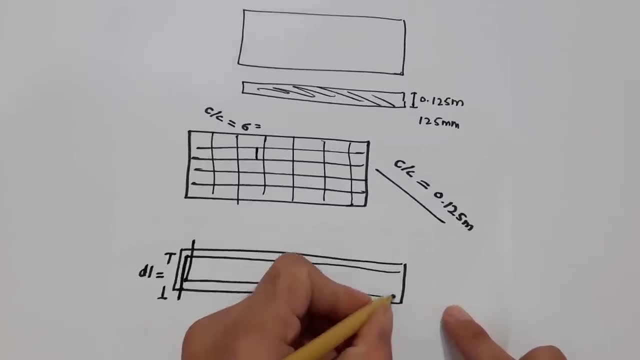 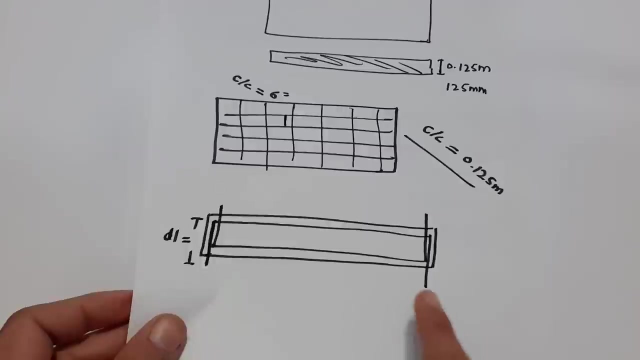 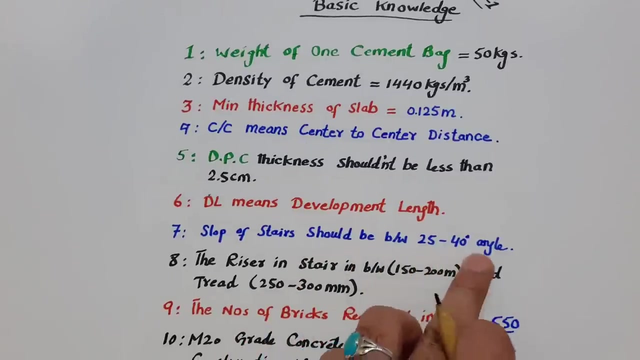 length is called this length. okay, from here to here this is called DL means development length. okay, so this is called development length, as you can see, which makes a good bond between steel and concrete. okay, so at the end we are providing these. the next one is, guys, seventh slope of steer should be between 25 to 40 angles. what? 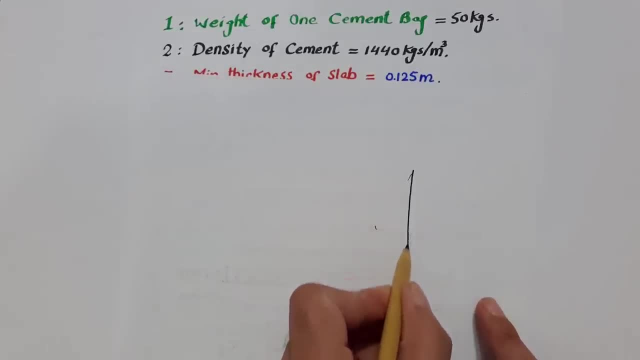 does. it means, guys, you can see, this is a wall, this is still okay. this angle: guys, you can see, these are steps, okay, so this angle should be between 25 to 40 degree. okay, it should not be more than 40 degree, otherwise the the people will face more problems when they are. 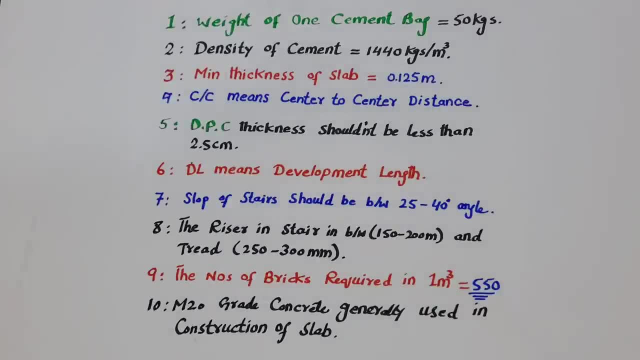 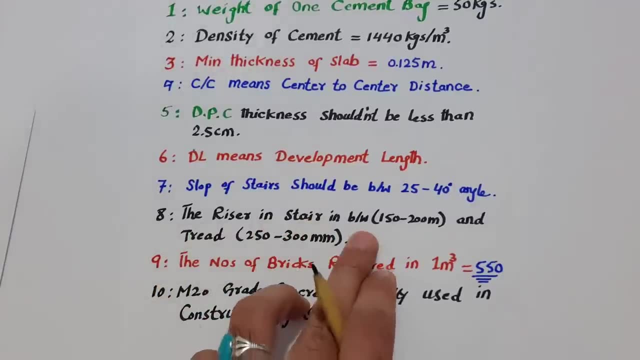 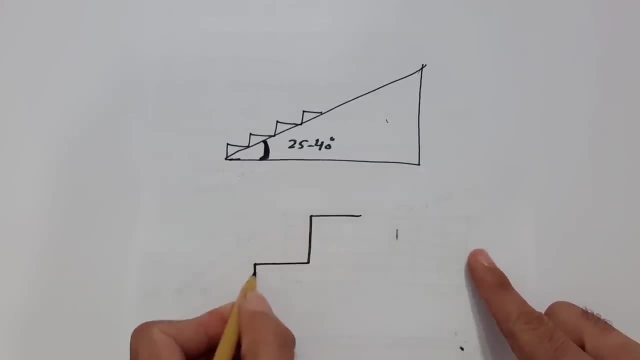 using these stairs. okay, so the angle should not be between 25 to 40 degree. next one: guys, you can see here at the riser and stairs in between 150 to 150, 100 riser mean, as you can see in the steps. okay, so you can see this is called. 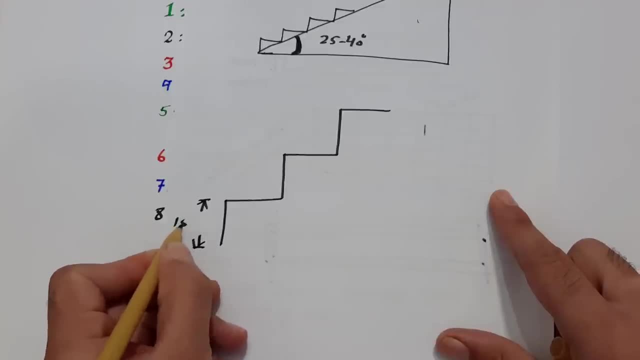 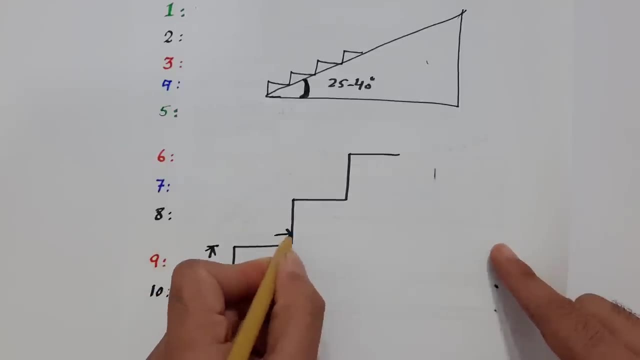 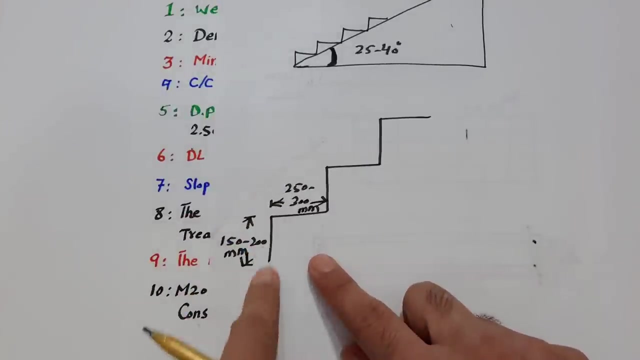 riser, so it should be between 150 to 200 millimeters. this height, okay. and the next one, this is called trade, this, okay, so the trade should be 250 to 300 mm. right, this one. so the one is riser, the vertical is riser, the horizontal is. 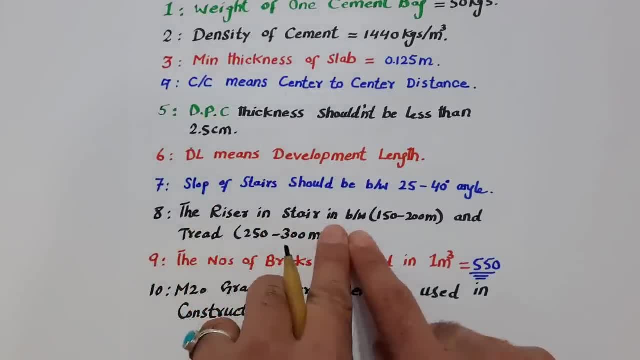 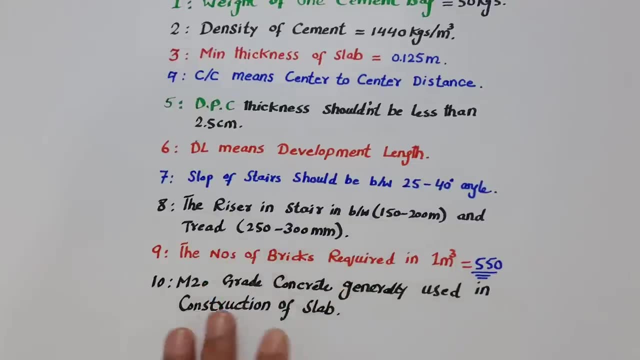 trade and steering. so it means the riser and steer is between and between 150 to 200 mm and the trade 250 to 300 millimeter. okay, this is very important, useful. the next one is, guys. ninth, the number of brakes required in one meter. 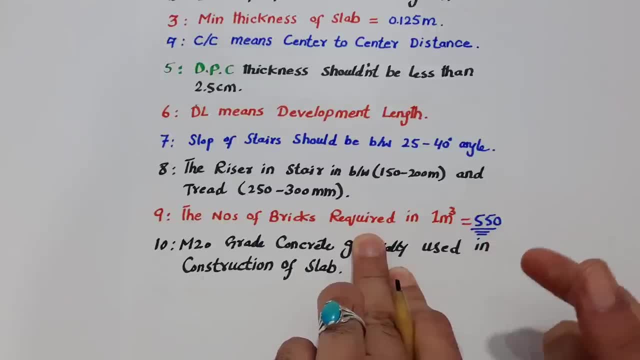 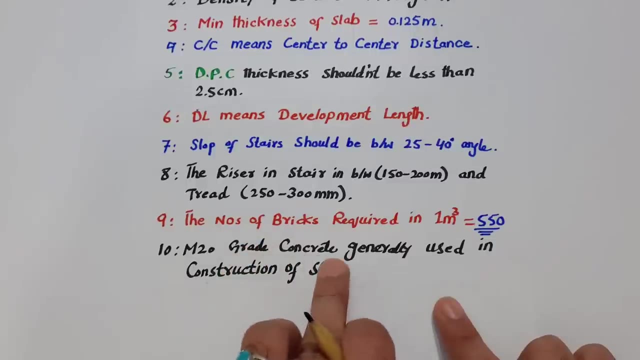 cube. anyone can ask from you how many numbers are required in one meter cube? okay, Okay, so 550 numbers of bricks are required in one meter cube. Okay, next one, guys. you can see M20 grade concrete generally used in construction, oxalate. 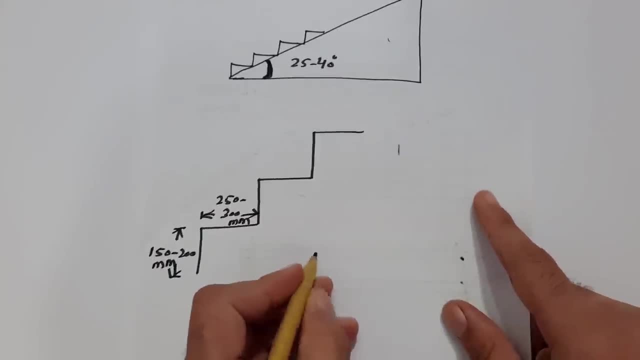 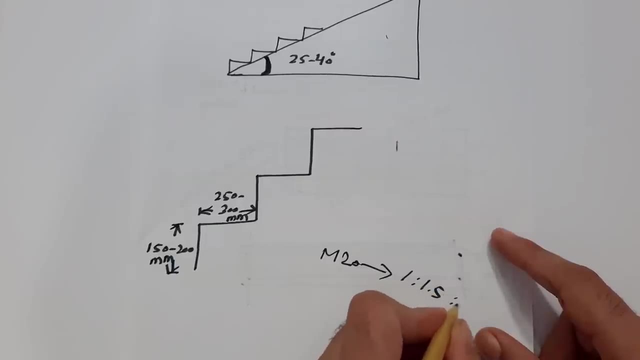 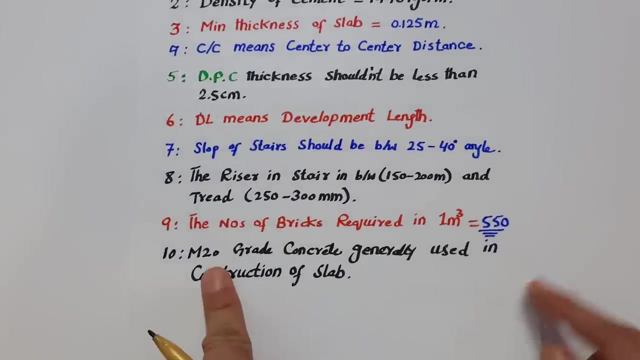 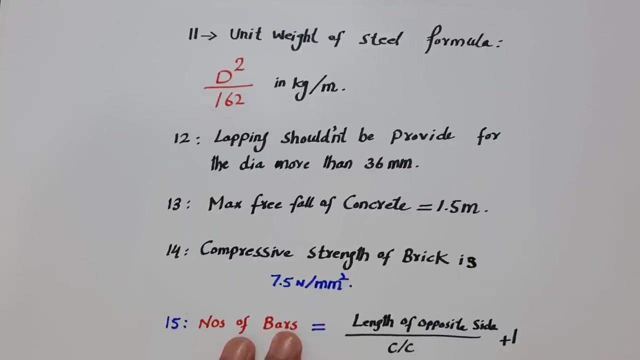 So what is M20 grade concrete? M20 means M20 ratio is 1.5, ratio, 3.. This is the ratio of concrete for M20.. So it's generally used for the construction of slab. Okay, guys, the 10th one is. the 11th one is unit weight of steel. 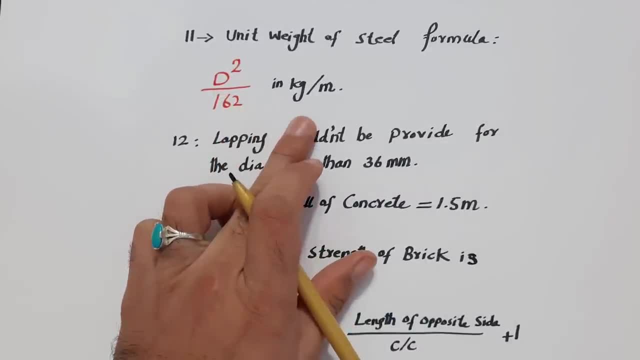 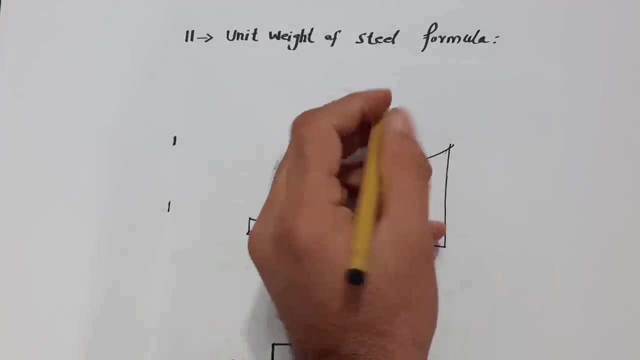 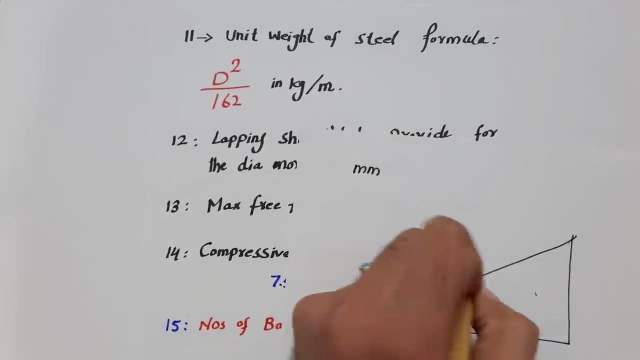 The formula is D square divided by 162 N kg per meter. This is weight of steel for one meter. So how you can find the total weight of steel? Okay, so guys, remember this. D should be N millimeter. Okay, For example, I'm using the formula: 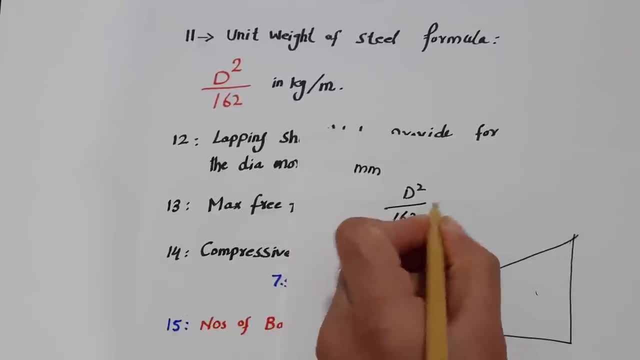 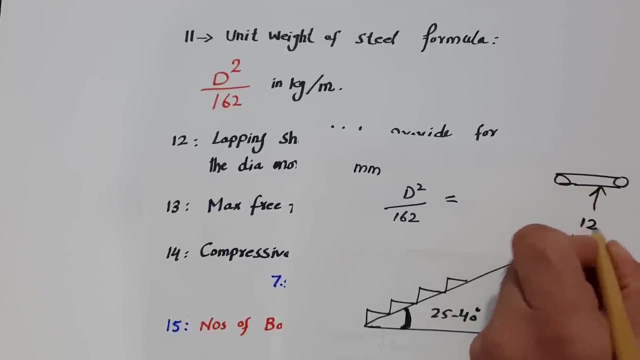 So which is D square divided by 162.. Okay, so is equal. For example, I'm using the dia. This is steel rod. Okay, which dia is 12 millimeter? Okay, so the formula will be 12 multiply 12 divided by 162.. 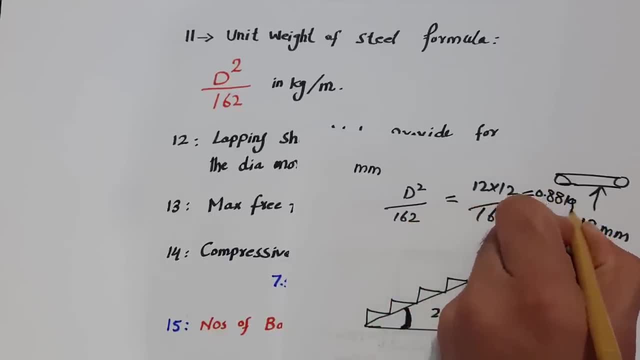 So it will become 0.88 kg per meter. So this is the weight of steel for 12 millimeter dia of steel. Okay, So this is the weight of steel for 12 millimeter dia of steel. So this is the weight of steel for 12 millimeter dia of steel. 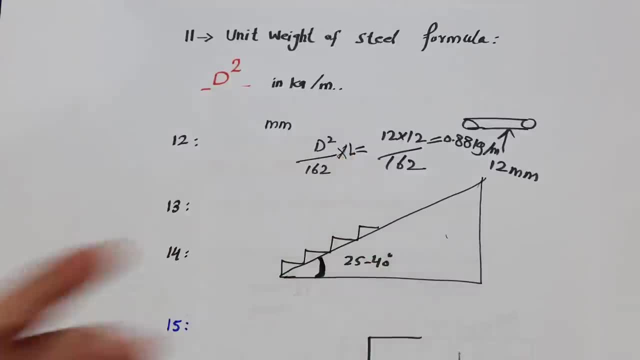 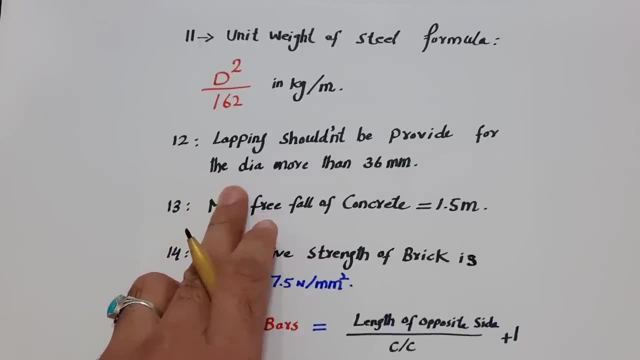 Okay, so with the running length you can also multiply. Right, That's the 12th. one is leaping. shouldn't be provided for the dia more than 36 millimeter. How, For example? guys, you can see this is a steel rod. 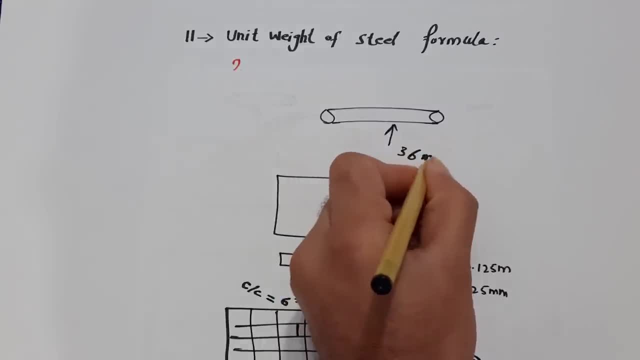 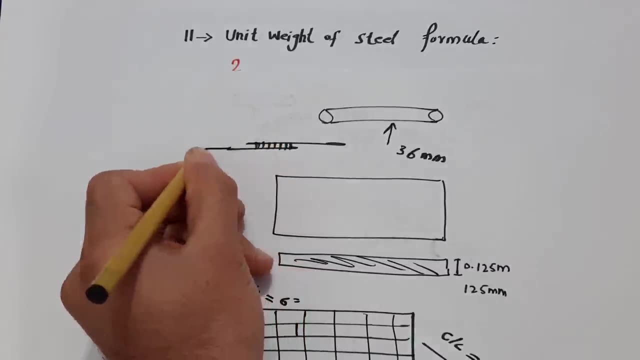 If the dia is more than 36,, 36 millimeter or 36.. So the leaping should not be provided. This is leaping guys, you can see. Okay, So the leaping should not be provided for this. Okay, less than this you can use. 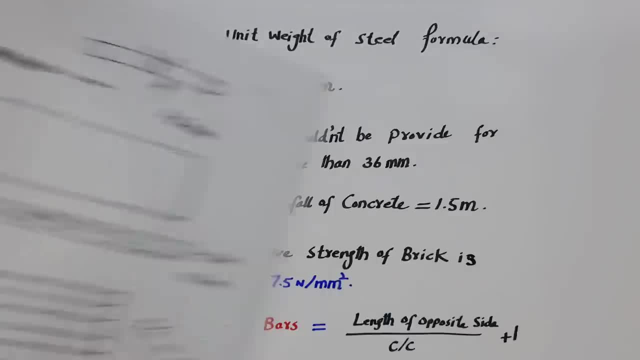 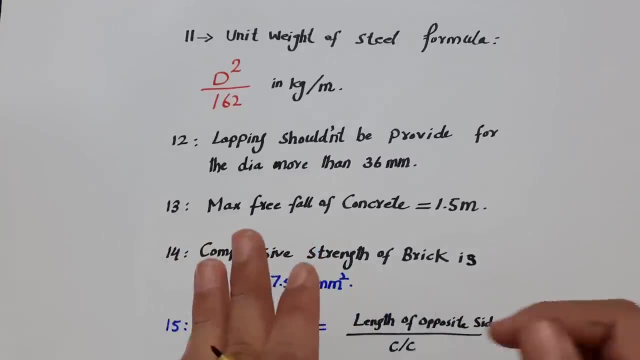 Okay So for this you can use the coupler method or any other one. Guys, the 13th one is mix pre-fall of concrete. Okay So, pre-fall of concrete. when we are using our during pouring of concrete and slab, or in any member, RCC member, we are providing the concrete. 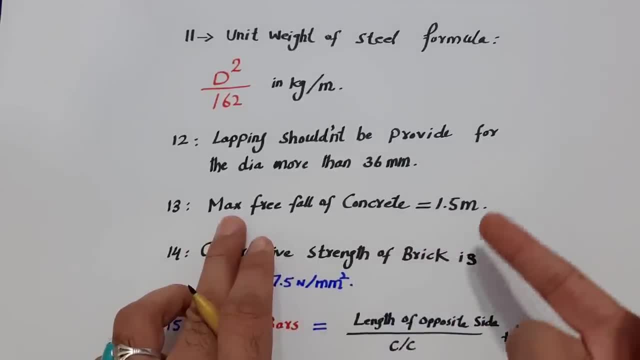 So the concrete height should not be more than 1.5 meters, So mix pre-fall should not be more than 1.5.. Otherwise it will make the bleeding segregation, et cetera, and you will face the problem.